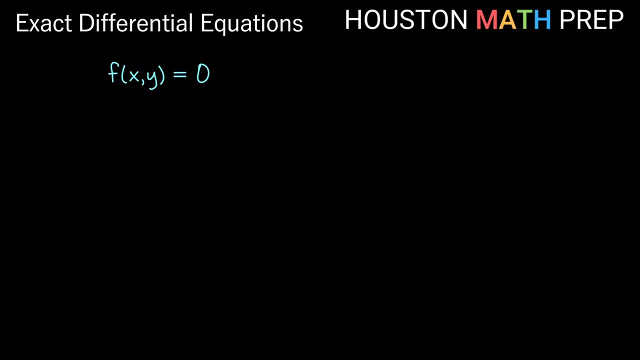 in calculus, multivariable calculus- if we had a function of x and y equal to zero and we wanted to take the derivative of that function with respect to x, then we actually need to use the chain rule to do this derivative And the first part of the chain rule, because f is a function. 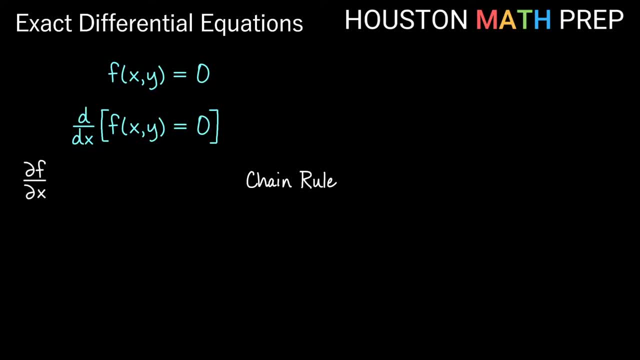 of x and y, we actually get partial derivative of f with respect to x times dx, dx, plus the partial derivative of f with respect to y times dy dx. Now, obviously on the other side, on the right side, we would still get equal to zero taking the derivative with respect to x. 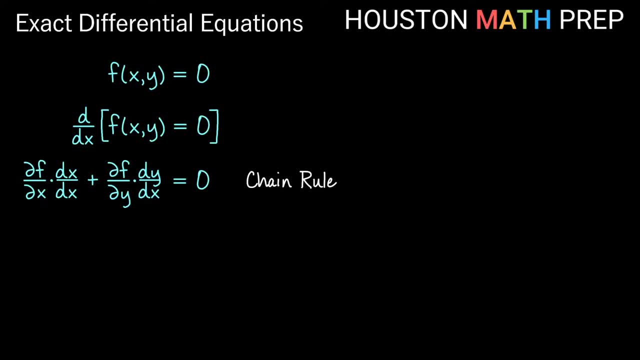 If we simplify these partial derivative notations to our subscript notation- and I call these partial fx plus partial fy, dy, dx- one shortcut that we might have developed at this point for working with derivatives would be move the partial fx to the other side and then go ahead and divide. 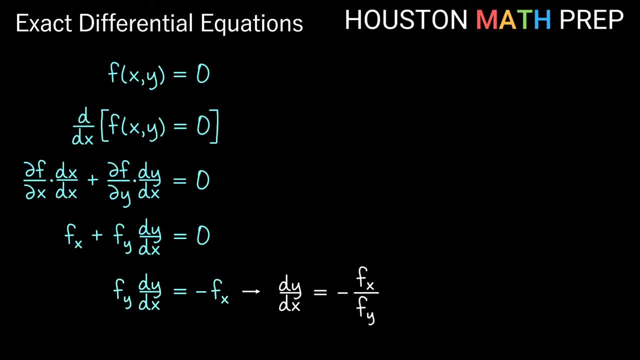 by partial fy and we get a nice shortcut. dy, dx is equal to negative partial fx over partial fy, And this is actually a shortcut For implicit differentiation. so let's go ahead and set our implicit differentiation shortcut to the side. Let's look at another operation on this function here, our function of fxy, and that's 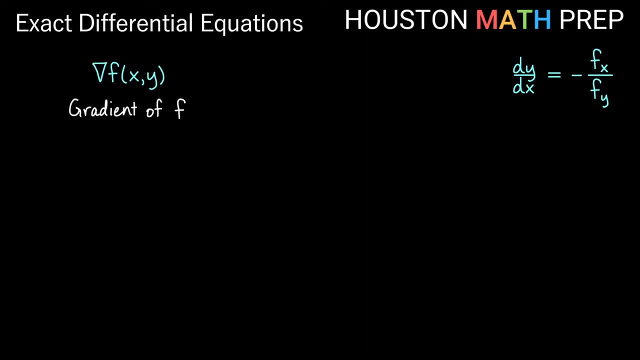 actually del f, taking the gradient of this function f. The gradient of f is an operation that gives us information in terms of a vector field, that gives us the vector partial fx, comma, partial fy, and that tells us information about rates of change on our surface. 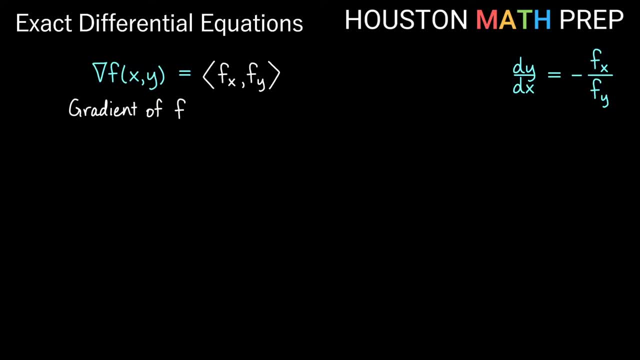 This function of x and y. When we think of this as a vector field- remember a vector field- we might think of some formula m comma, some formula n, and that's just a formula for vectors anywhere in the plane. One thing: you might have asked yourself about a vector field if you've done these before. 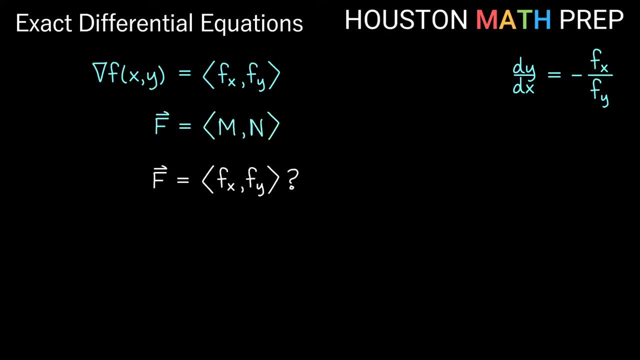 is wanting to know: is my vector field f a gradient of some function? In other words, we're asking: is m partial fx for some function and is n partial fy for that same function? How would we know if that's true? Well, we think about mixed partial second derivatives and remember the idea is: 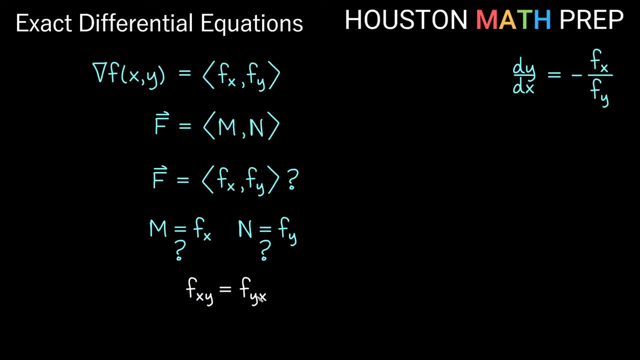 these mixed partial second derivatives should be the same as long as the function is continuous and well behaved and all that stuff on some region. Now, partial fx, if I take the derivative with respect to y, gives me fxy, and partial fy if I take the derivative with respect to x. 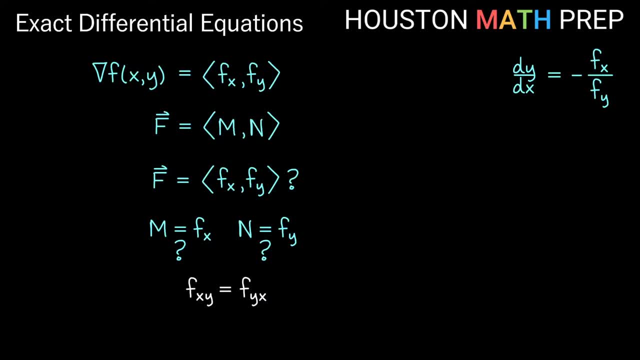 gives me fyx, and those are supposed to be equal to one another. So what that says is: if I take the partial derivative of m in my vector field with respect to y, I take the derivative of fx and the partial derivative of n with respect to x in my vector field, if those are equal to one. 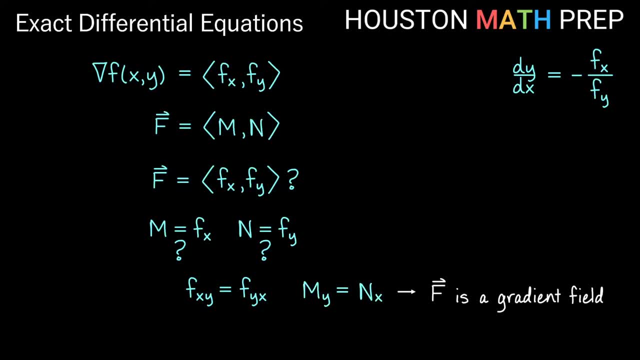 another. then I get that my vector field is a gradient field and that tells me lots of other things that provide me shortcuts for all sorts of integrals that I can do with vector fields. This condition of the partial derivative of m with respect to y equaling the partial derivative. 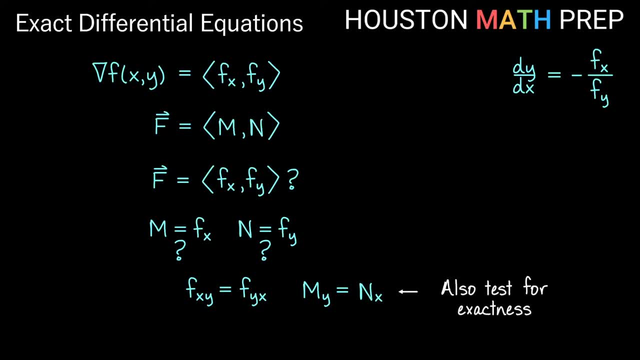 of n with respect to x is also our test for exactness, to determine if something is an exact first order differential equation. So if M is Fx and N is Fy, let's go ahead and plug that information into our implicit differentiation statement that we know is true. That would give us 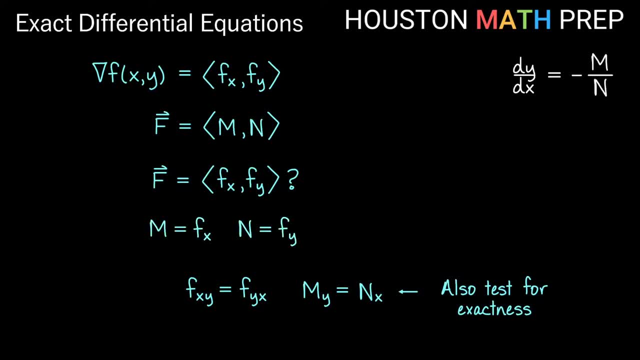 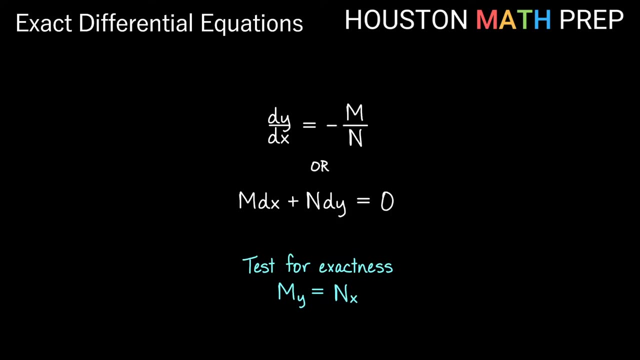 that dy dx is equal to negative M over N, And this begins to look like a differential equation that we might see. This can also be arranged a little more nicely to see what M and N are specifically, so that they're not in the fraction. with some sign changes here, We can rearrange this as MDX plus NDY. 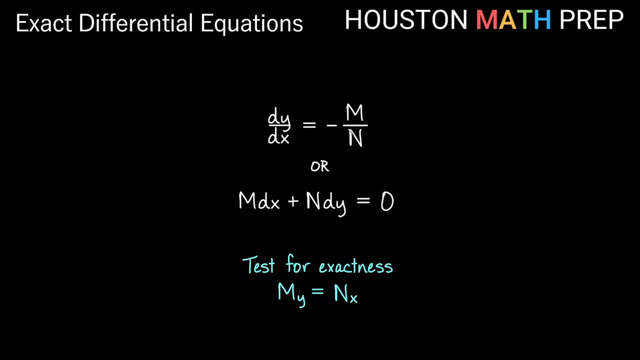 is equal to 0, and the way we'll test to see if this is an exact equation here is, just to check, does the partial derivative of M with respect to Y equal the partial derivative of N with respect to X? So if our equation is exact in, 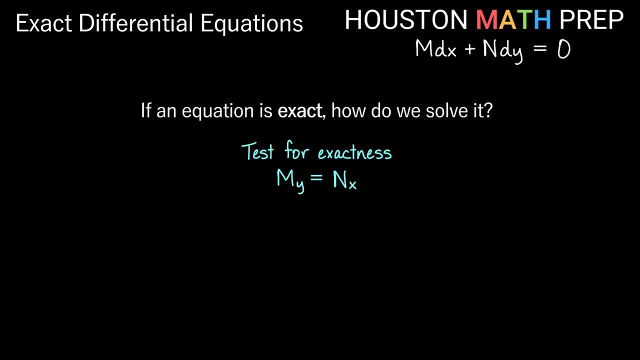 other words, it passes our test for exactness. what do we do to solve it? Well, remember that M is partial Fx of some function and N is partial Fy for some function, and that's what our test for exactness says. So what we need to do is 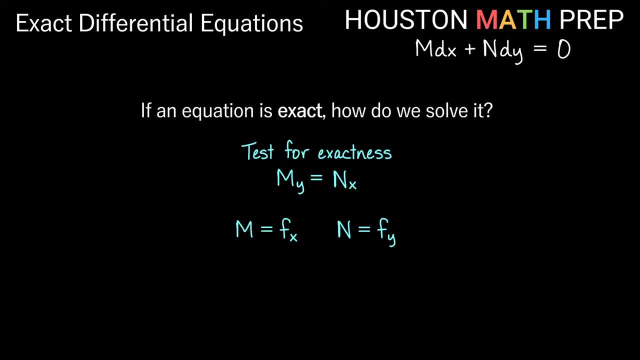 just undo the equation and we'll see what happens. So let's go ahead and plug that into the processes that got us this M and N, and we can find dy, dx. In other words, I need to undo the derivative with respect to X for this one and undo the. 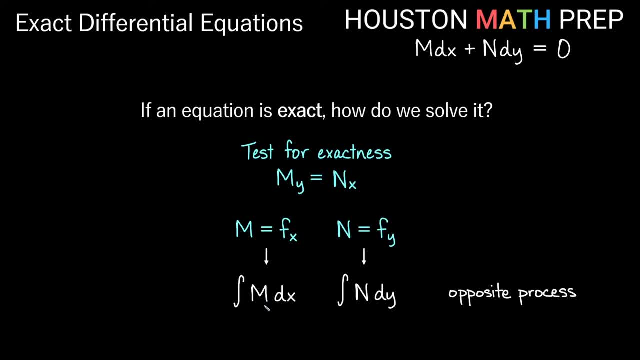 derivative with respect to Y for this one. So I will integrate M with respect to X and I will integrate N with respect to Y. And if you did this in calculus 3, this was about finding something we called the potential function, And it's. 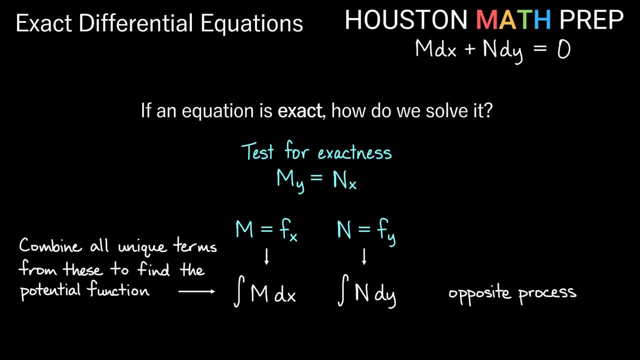 really a similar idea in how we will solve our differential equations when they are exact, first-order differential equations. Remember that the first order differential equations are the ones that we need to solve. Remember that the first order differential equations are the ones that we need to solve. 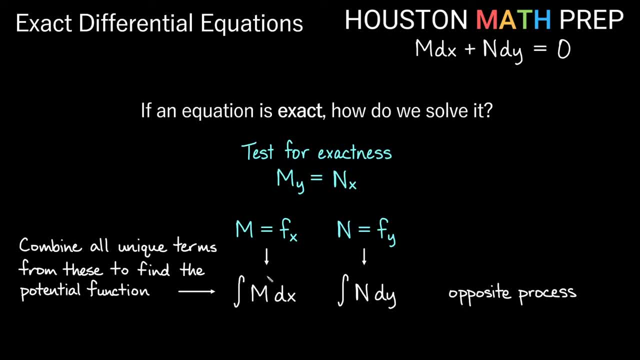 Remember a short way to view the method of finding the potential function from calculus was to combine all of the unique terms that we get from both of these antiderivatives. that gave us the potential function, and here it will actually help us find the solution for our exact differential equation. 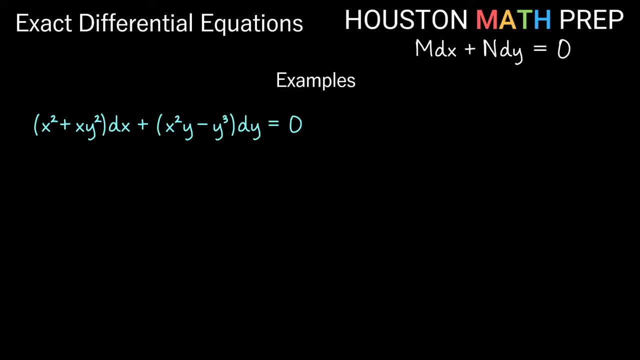 We'll go ahead and work a couple of examples for you here. First we'll test if they are exact, and if they are exact we will solve them. And we'll check for exactness on the first couple using this form and then we'll actually set them up. 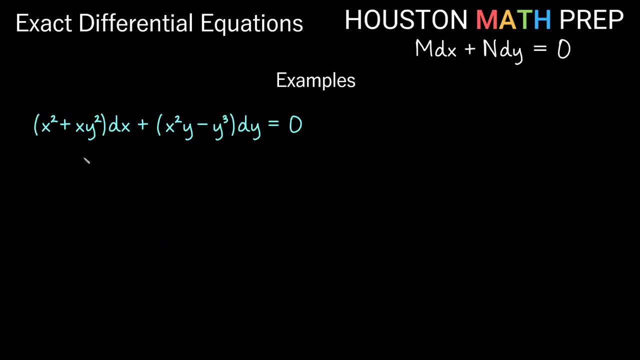 as dy dx equals and do a couple of those. So here we've got X squared plus XY squared times, dx plus X squared, Y minus Y, cubed dy is equal to 0. so this here is my M in this one and this is my n. 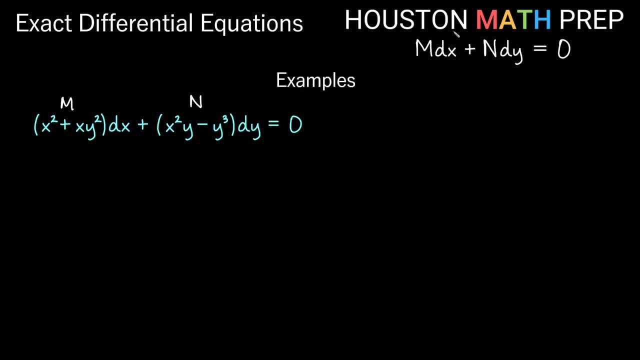 Alright, you can see it's set up as MDX plus ND, Y equals 0, so I should just be able to check here. so let's go ahead and do that. So let's check what is the partial derivative of M with respect to Y. Now we treat X as a constant, remember. 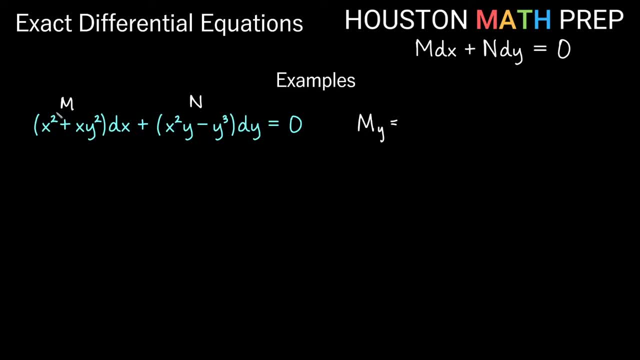 taking the derivative with respect to Y, respect to y, So this x squared term is really a constant, so we get zero from that. Taking the derivative of xy squared, thinking of this x as just some constant multiple, the two will come out front and we'll actually get 2xy. If I look at the partial derivative with respect to x, of n, 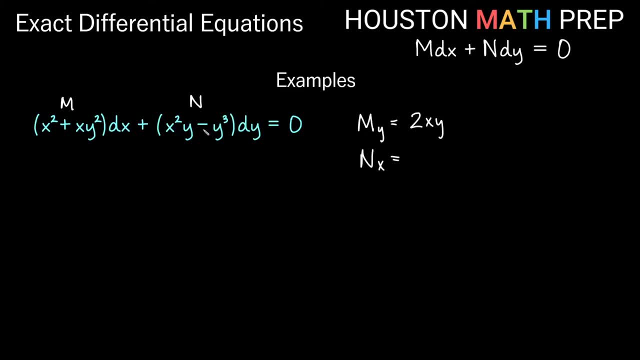 I go ahead and take the derivative with respect to x of this here, treating y as the variable and x is the constant. now, So if I treat x as the variable, this 2 comes out. we get 2x. we keep the constant multiple y, we get 2xy. The derivative with respect to x of y cubed. 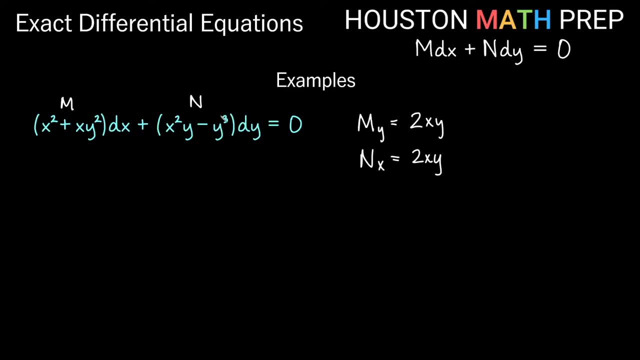 since it's with respect to x. y, cubed would be a constant, so the derivative of this term is zero, And you can see here these are equal to one another. so we know partial my equals, partial nx, and this is in fact an exact equation. 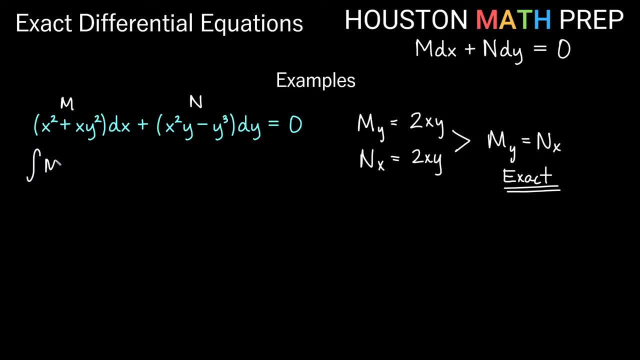 So, to find our solution, we're going to need to find our solution. So, to find our solution, we're going to need to go ahead and integrate m with respect to x, and we'll also integrate n with respect to y. We'll 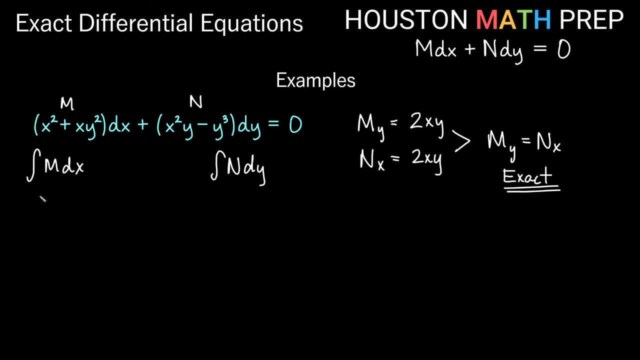 combine all of the unique terms that we get from both of these into our solution. So our integral mdx is going to be integral of x squared plus xy squared dx. Now, treating x as the variable here, we would get one third x cubed plus. 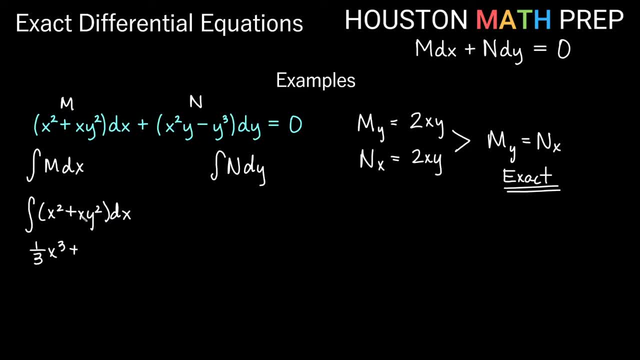 this is just a constant multiple, so we keep the constant multiple. Power goes up by one. here we'll get one half. Power for x goes up by one, so we get x squared, y squared, plus some constant, And because we're integrating with respect to x and 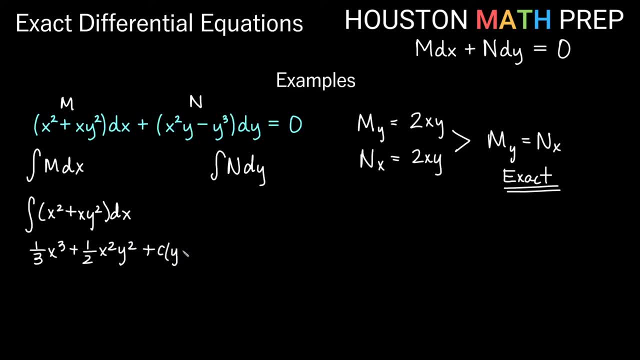 treating y as a constant. technically this constant could depend on y. What this is really saying here is that in the other piece of this we might get some terms that only involve y. Let's do this other antiderivative here, so the integral of n, dy. 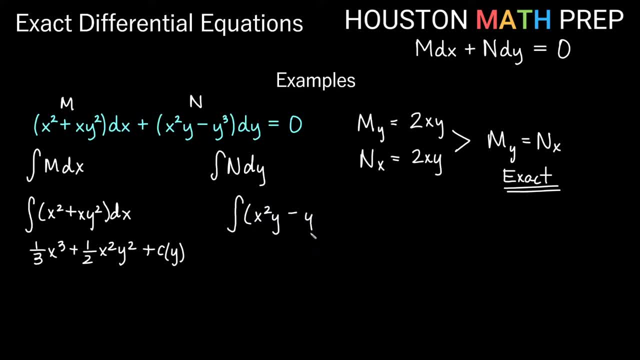 is going to be the integral of x squared y minus y cubed dy. So if we integrate with respect to y, treating x as a constant, This is a constant multiple x squared. here. Power goes up by one for the y we divide by two. 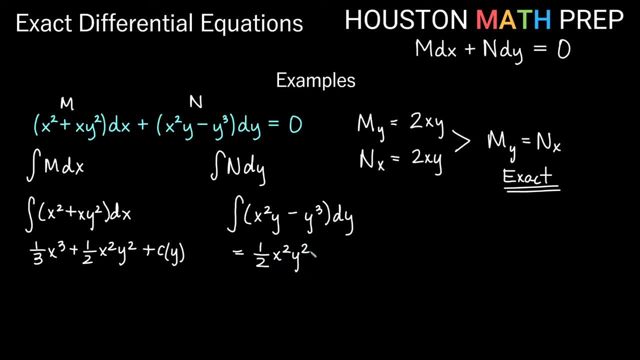 so we get one half x squared, y squared minus anti-derivative of y, cubed with respect to y, would be one fourth y to the 4, plus some constant. Now technically our constant could depend on x and this is really saying that in your other statement you might have some terms. 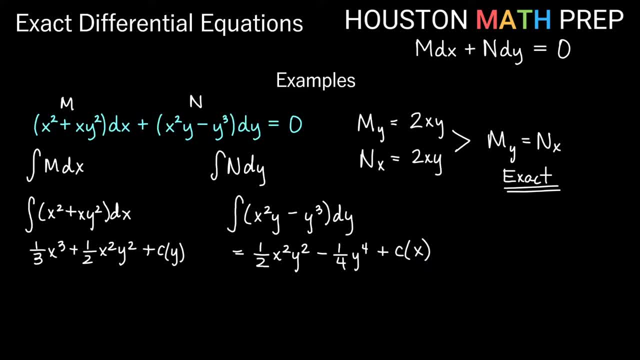 that are only in terms of x, and you can see that right. And if you look at all of our unique terms, you can notice over here, this c maybe depending on y that we're talking about is actually this term that only has y in it, and this c maybe depending on x over here is actually referring to this. 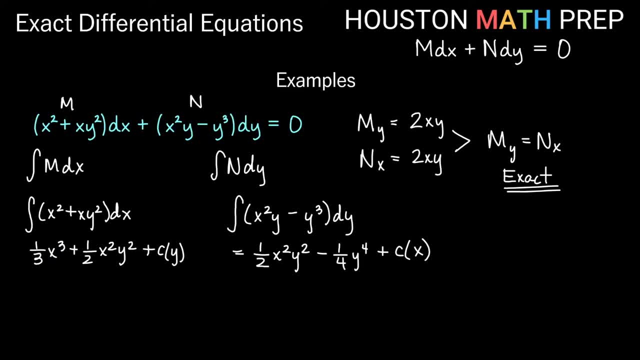 one-third x cubed, that only has x in it over here. So if we combine all unique terms here and we set that equal to just some constant, then we'll go ahead and say our answer is one-third x cubed, so that takes care of that term, plus one-half x squared, y squared. that takes care of both this. 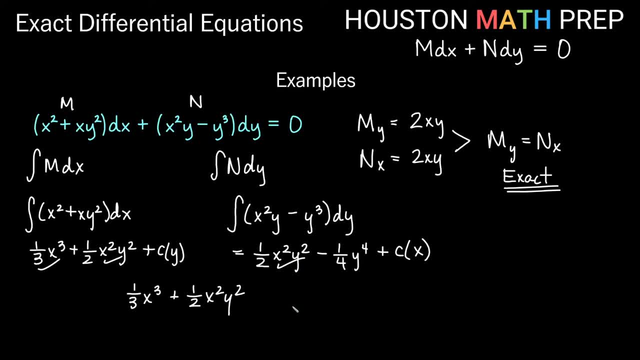 term and this term. we don't write that term down twice. we only take unique terms minus one-fourth y to the four. so that takes care of that term. now, everything is taken care of, except our constants. so we go ahead and say: equal to c and that is equal to c. 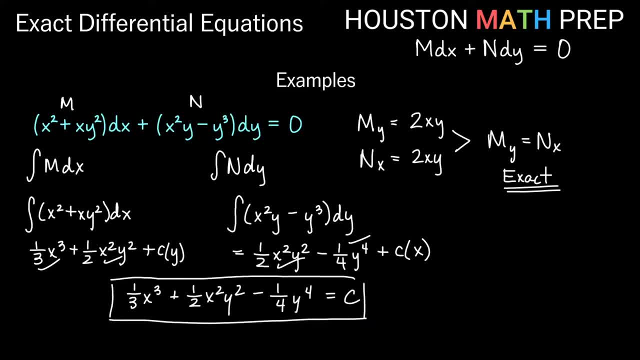 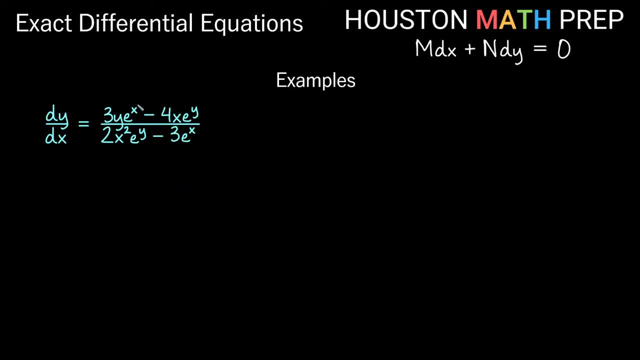 This is our solution for this exact equation. Let's do one last one. this one is exact, we'll go ahead and show you. so we have dy. dx equals three y e to the x minus four x e to the y, all over two x squared e to the y minus three e to the x. so we'll go ahead and first get rid of denominators, so multiplying. 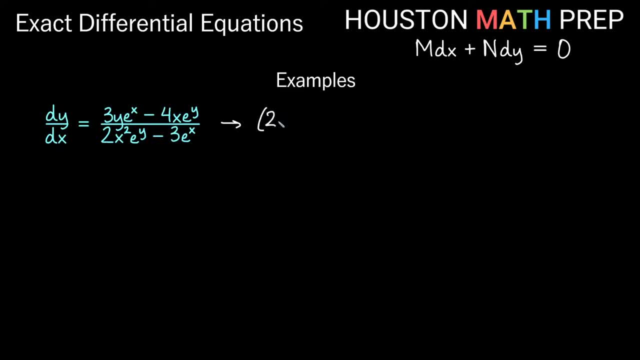 this to the other side and dx to the other side, we'll get two x squared e to the y minus three e to the x. dy is equal to our top here. three y e to the x minus four x e to the y times dx. let's go ahead and move our dx term over to the other side, so getting that on the 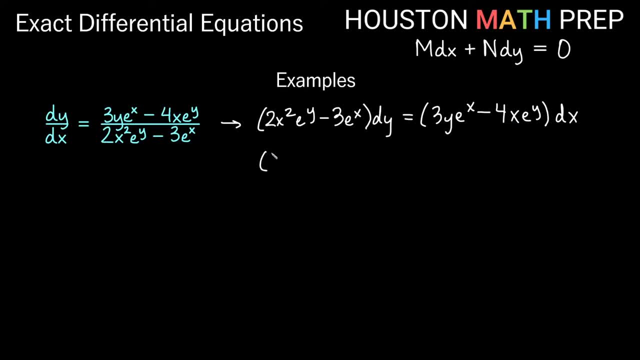 other side. it would change signs, so this negative term becomes positive. we'll say four x e to the y. this will become negative. so minus three y e to the x- dx plus exactly what we have there. we didn't move our ndy at all. so two x squared e to the y, minus three e to the x. 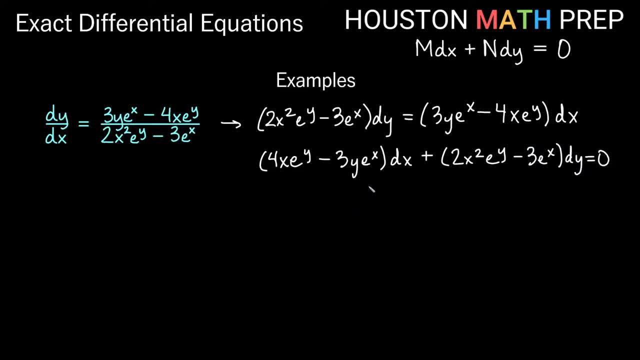 dy is equal to zero. so now let's check for exactness. you'll see that this works out partial m y- this is our m here- derivative with respect to y of the first term would keep our e to the y and our constant multiple would stay. so this is four: x, e to the y. 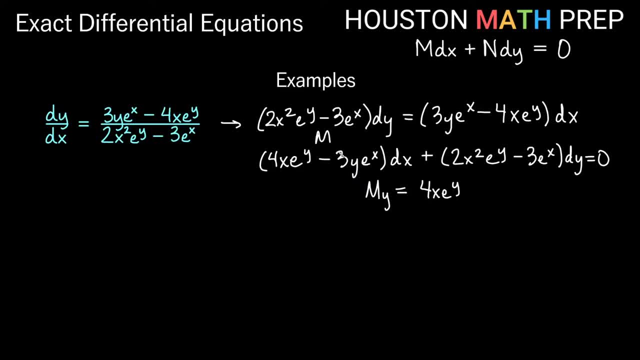 derivative with respect to y. here the negative 3 e to the x is all a constant multiple, so the y just drops off. we get minus 3e to the x. looking at n over here and finding partial n- x, then the derivative of this first thing with respect to x, we would get a 2 coming out. we'd get 4x e to the y. 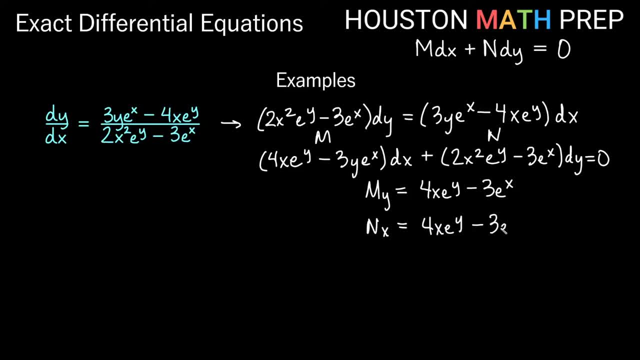 and the derivative with respect to x. there is pretty basic minus 3e to the x. you can see that that these are equal. So since m y equals n x, then we get that this is exact and remember what we do once we find that We figure out the antiderivative of m with 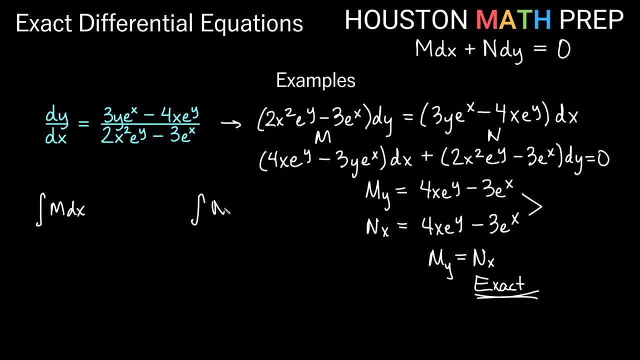 respect to x. We figure out the antiderivative of n. with respect to y. We find all unique terms. We combine them into our solution equal to a constant. Okay, so this one first. here we'll take the antiderivative of Now go ahead, and. 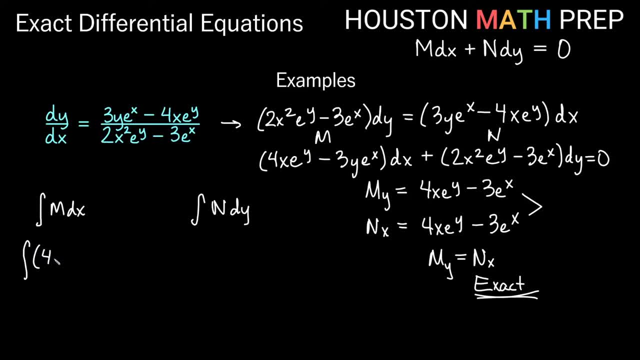 do it from this form, actually seeing what m is, That is, 4 x, e to the y minus 3 y, e to the x, dx. So let's go ahead and do that and give myself some room here. So if we're integrating dx, think about this. e to the y is just part of the. 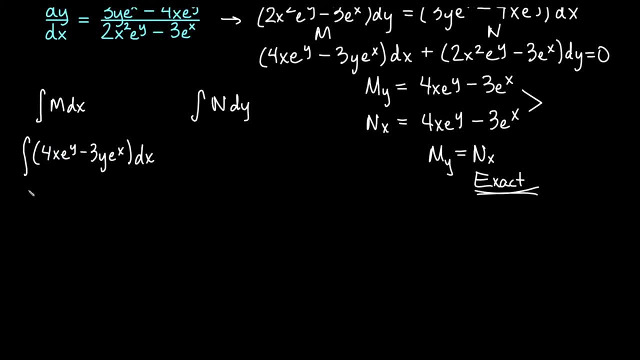 constant. So the power goes up by 1. here We divide by that power. So dividing by 2 will give us 2 x squared e to the y. Now e to the x is the part that has variable x in it. This negative 3y is just a constant. So we go ahead and say: 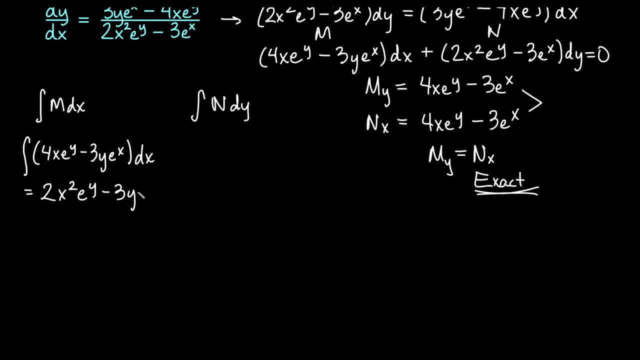 we keep the negative 3y and the antiderivative of e to the x is still e to the x. We get 2x squared: e to the y minus 3, y, e to the x plus some constant. that may also be a term with only ys in it. I'm going to go ahead and move my. 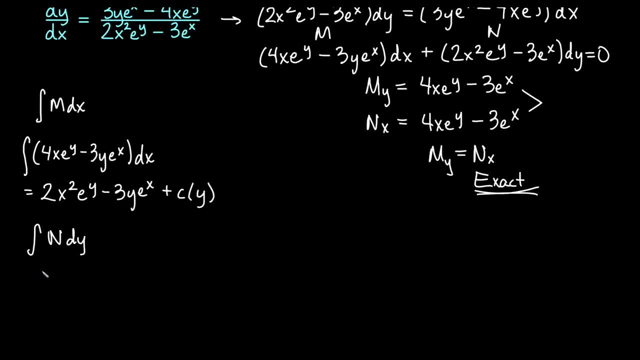 integral of n dy down here, so I have a bit more room. So we'll say that's the antiderivative of Here's our n over here, two x squared e to the x squared, e to the y, minus 3 e to the x dy this time. So if we integrate this with respect to y, 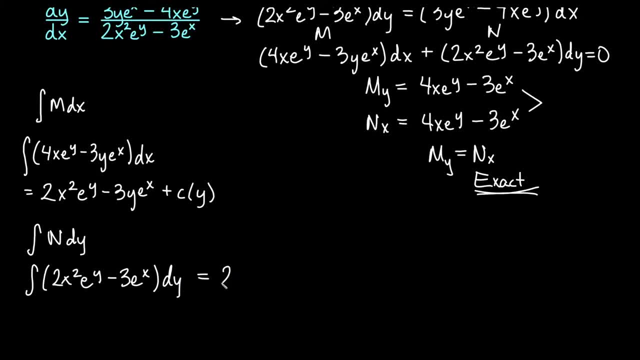 this is all a constant. multiple e to the y would stay itself. so we get 2 x squared e to the y and then, integrating this with respect to y, all of that's just a constant. so if I integrate that with respect to y, I get that thing times y. so we get 3y e to the x plus some constant. 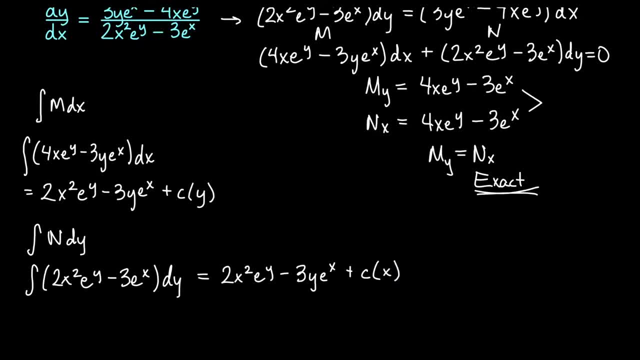 that may also involve terms only that have x in them. So we go ahead and look here at the unique terms that we have. I have a 2 x squared e to the y here and here, so that's part of my answer. 2 x squared e to the y, so that takes care of this and this, and you'll actually notice.